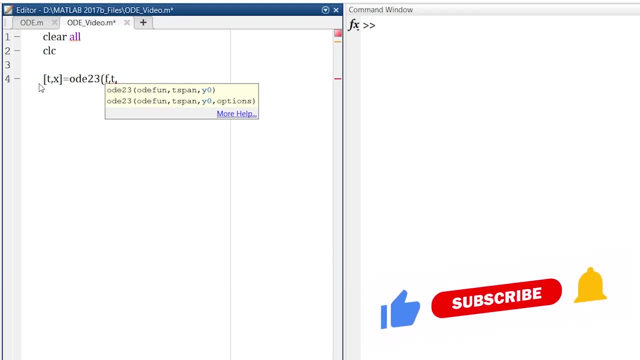 So, and then the initial condition. What would be the initial condition of x? Let's say, our initial condition is 1.. So this is the equation Here. we have not define the time span and functions in both equations. So what we will do, 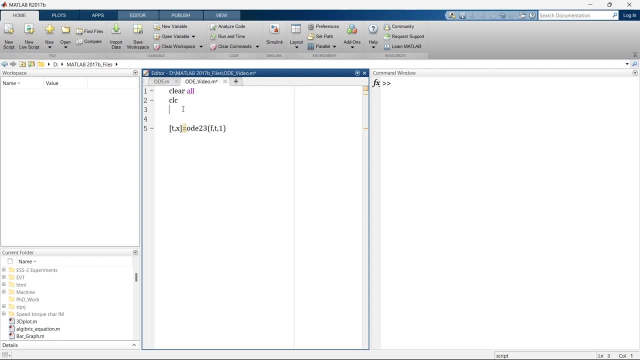 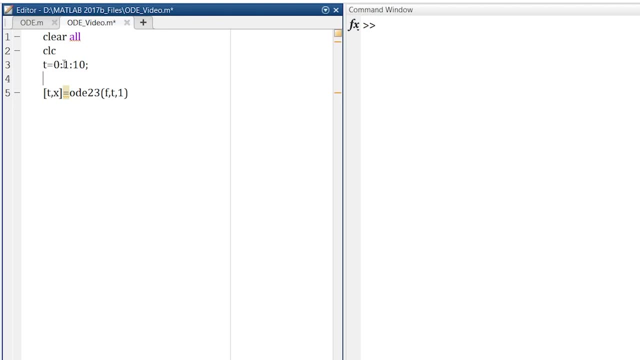 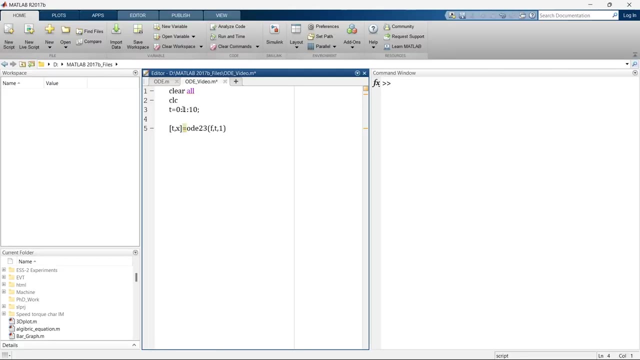 Before this equation: before the equation will define time span and equation. so let's say this is our time span and now I'm going to define the equation. there are various methods to define equation. one of the simplest method is inline equation: defining equation in line for. 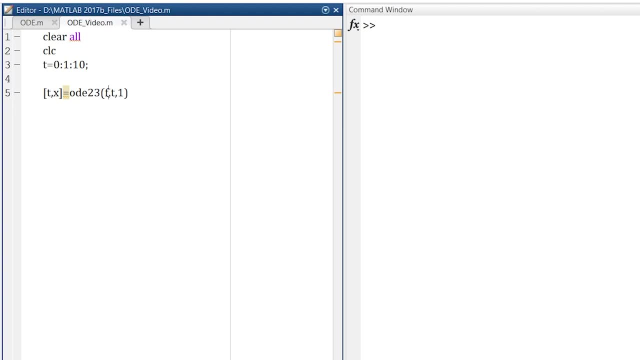 that we'll write what is our equation. our equation is F, so we'll write: F is equal to. we have variable T and X, so F is equal to add thread T, X. and now into this bracket we'll write our equation and the equation is 2 minus X square. so 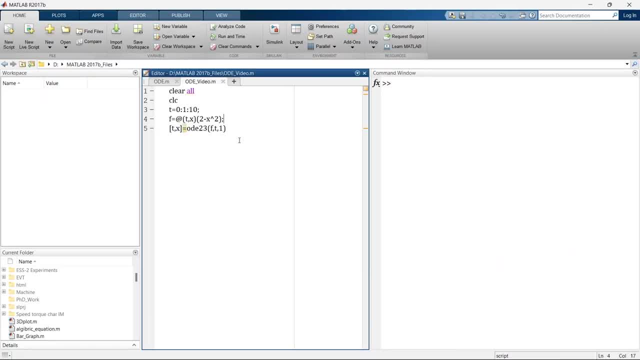 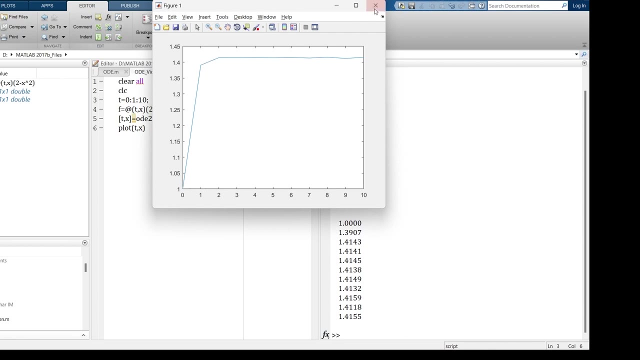 there we go and now we'll save it and run it. and these are the different results of differentiation. now let's plot these results in to the graph. if you want to have smooth curve instead of the slanted lines, then here you increase number of points and then you can have a smooth line. so this: 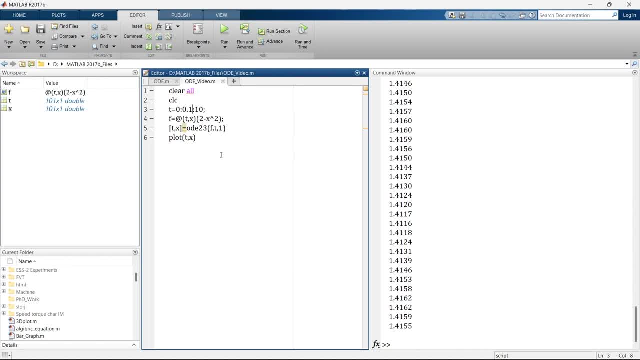 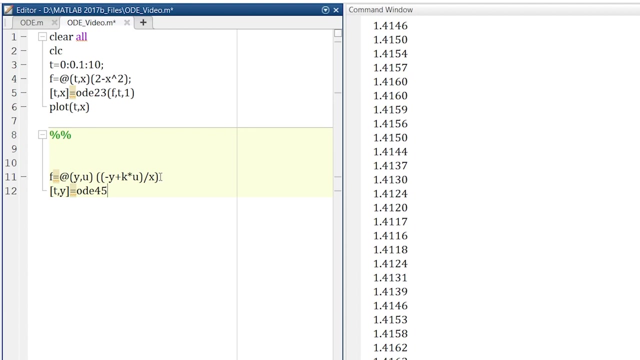 is one of the way of solving ordinary differential equation. now I'll show you some another method now. for example, our equation is minus Y plus KU by X- this one- and we solve it little bit differently. so we'll write OD equation for this now. instead of OD 23, we'll go for OD 45. now, first we need to define OD function. 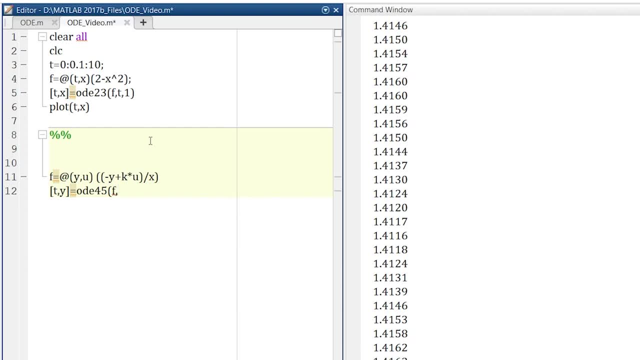 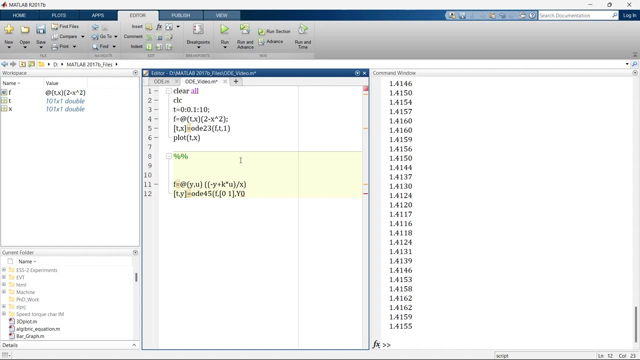 let's say our function is f. now we'll define time span. now, here we will define it little bit differently, will say 0 to 1 comma, and now we need to define the initial value, y0.. I can directly put the y0's value, or I can take this as a variable and then